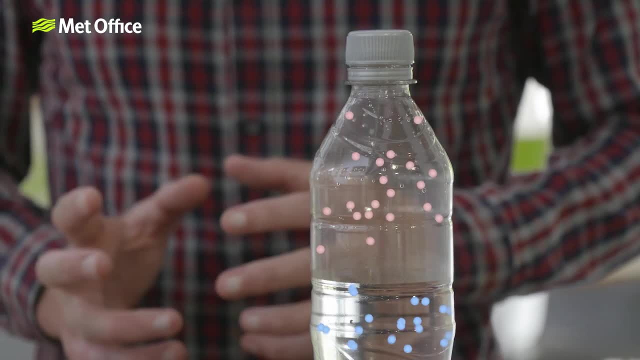 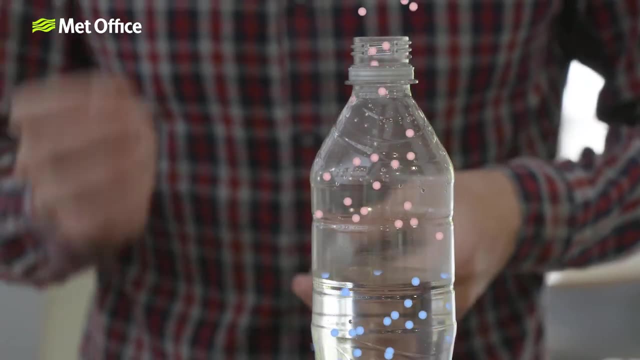 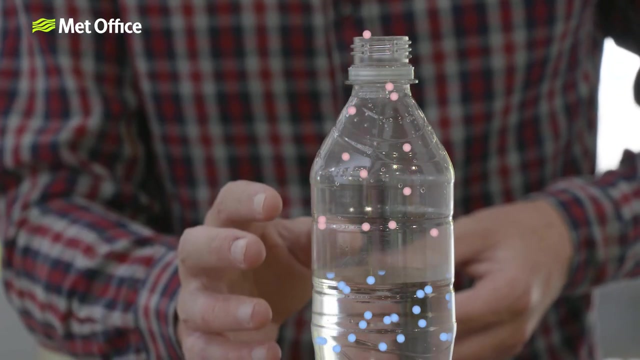 An equilibrium is reached If I remove the lid and heat up the water so that it's now warmer than the air. its molecules move around faster and more of them will escape. There's an increase in evaporation, whilst condensation remains the same. 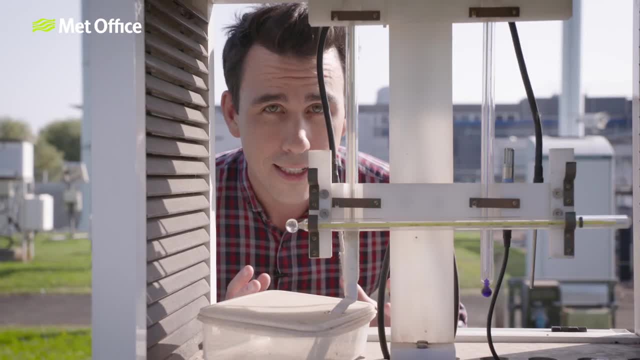 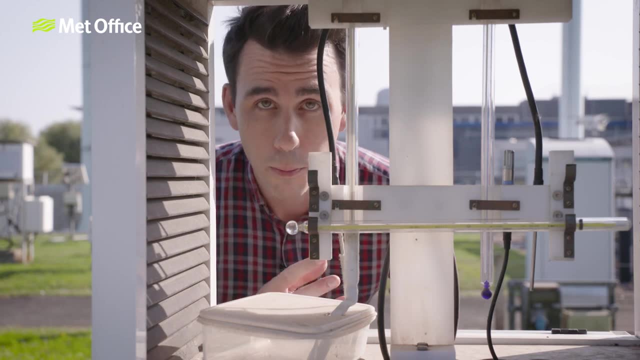 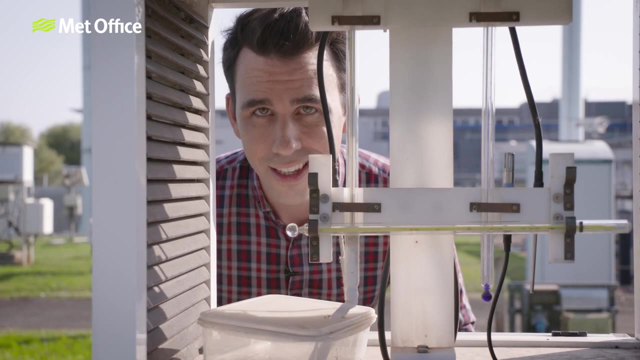 Back to the wet bulb thermometer. At first it has the same temperature as the dry bulb thermometer, but evaporation from its wet bulb causes it to cool down. As the wet bulb cools down, its rate of evaporation slows down until the rate of evaporation and condensation are the same. When the air is dry, there simply won't be as much condensation, so it will take more evaporative cooling for equilibrium to be achieved. The drier the air, the lower the wet bulb temperature compared to the air temperature. When the wet bulb temperature is the same as the air temperature. 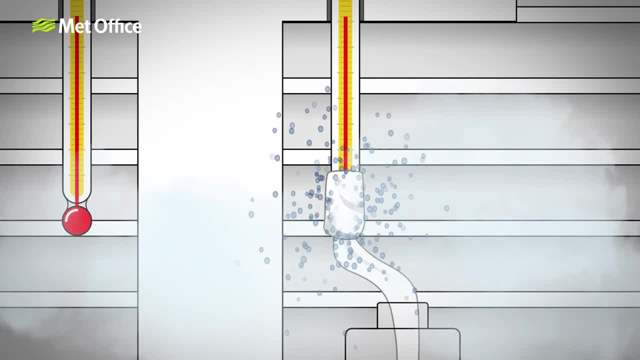 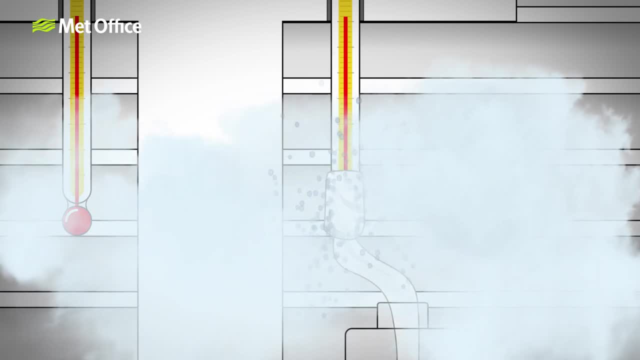 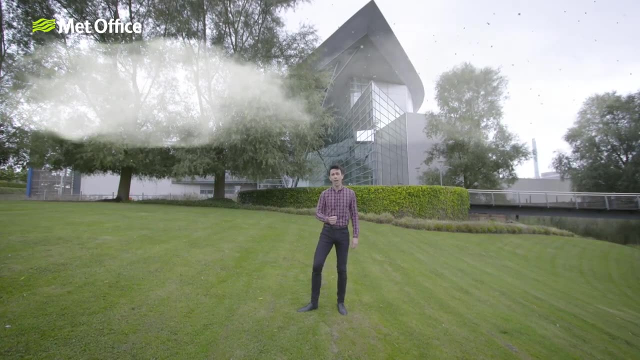 the rate of evaporation and condensation are already equal, The air is saturated and we say that the air has 100% relative humidity. Tiny water droplets will start condensing onto any surface, for example specks of dust in the sky above us to form clouds. 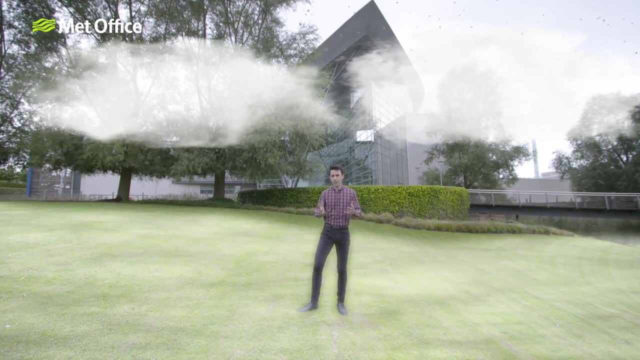 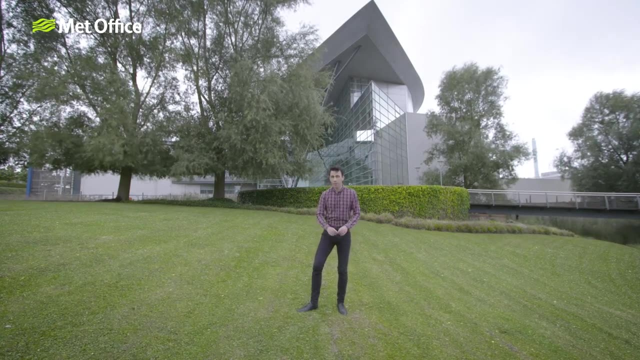 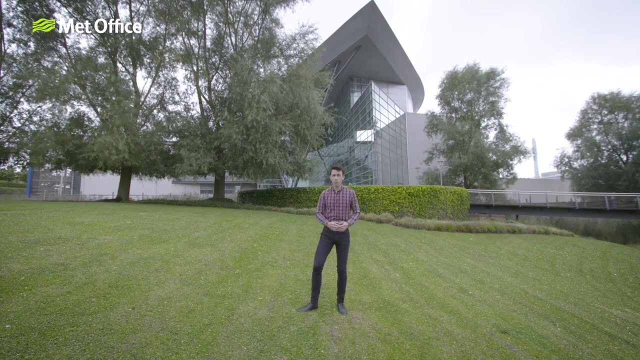 or fog if it's the air near the surface that is saturated, or dew if it's the air near the ground that has 100% relative humidity. In fact, the dew point temperature is the temperature the air needs to be cooled to for dew to form, for example, when the temperature drops overnight. 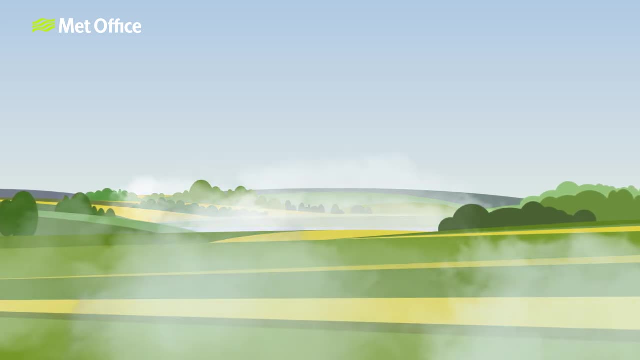 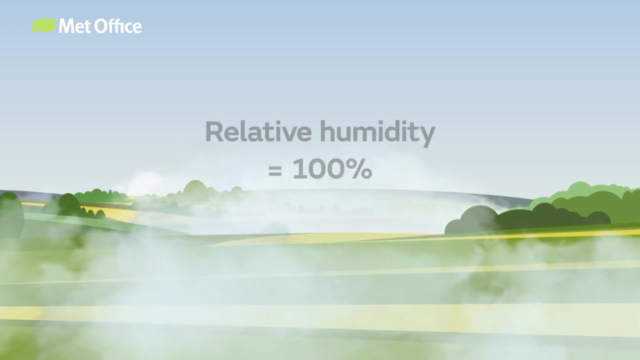 Just like the wet bulb temperature. when the dew point and air temperature are the same, the air has 100% relative humidity. It doesn't mean it will feel humid. A dew point of 5 Celsius won't feel humid at all, whatever the relative humidity. 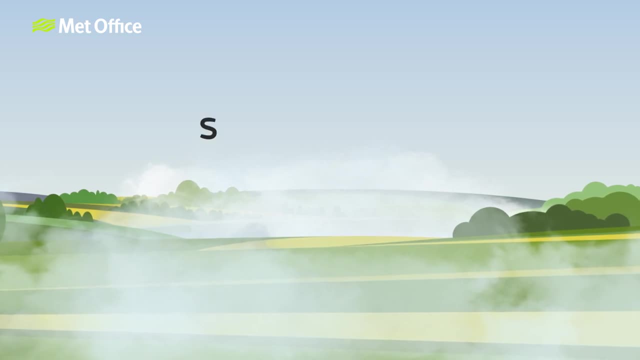 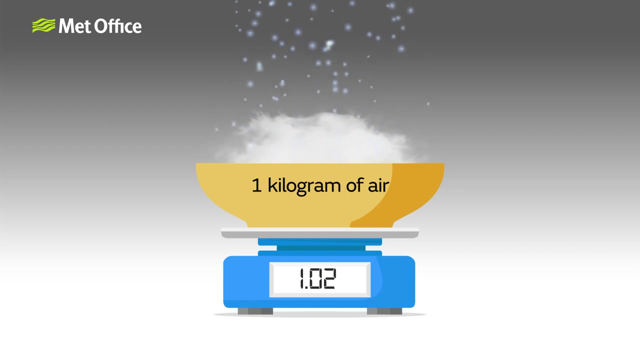 That's because there's another definition of humidity: specific humidity. This is simply related to the amount of water vapor in the air, for example, how many grams of water vapor per kilogram of air? The more water vapor in the atmosphere, the higher the specific humidity. 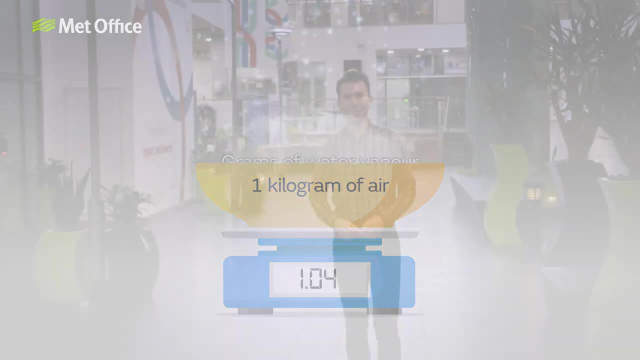 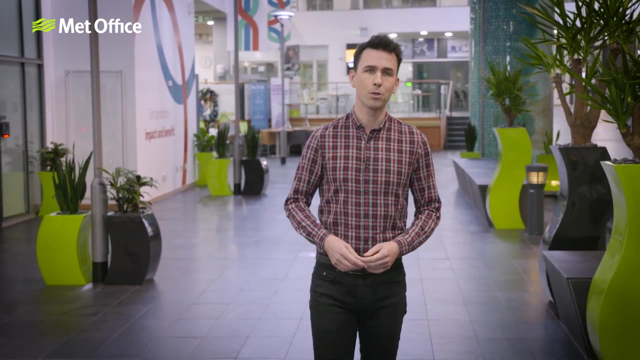 and the higher the dew point. How high the dew point needs to be for it to feel oppressively humid is subjective. It will depend on lots of different factors, including the kind of climate you're used to. For example, if you're used to the climate of the UK, 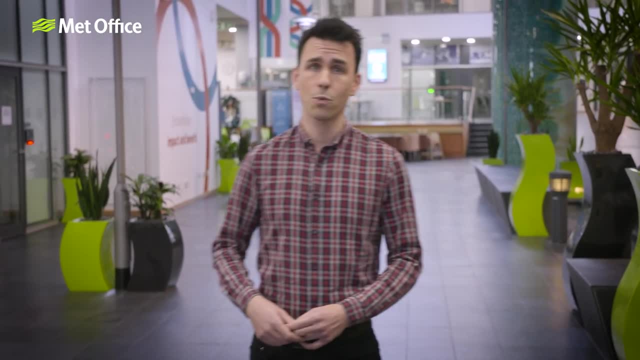 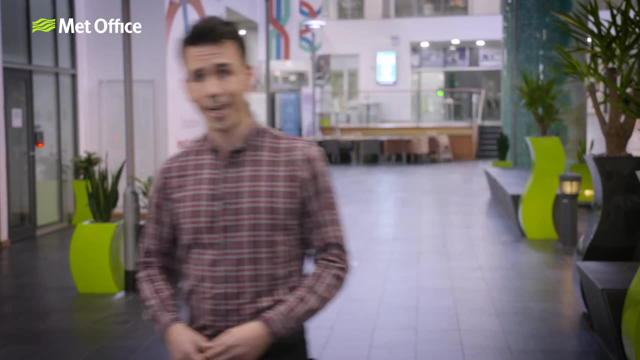 anything higher than a dew point of 15 Celsius may make you sweat. And how high does the dew point need to be for a bad hair day? Well, we'll let you be the judge of that.